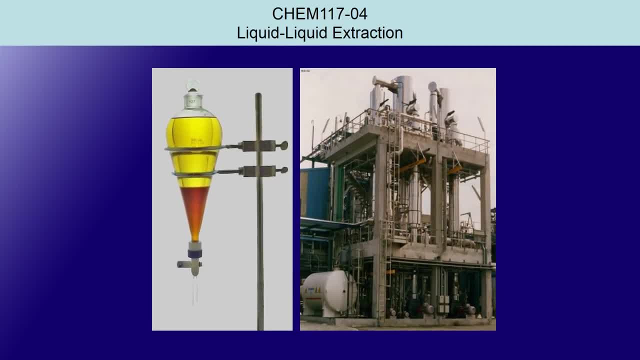 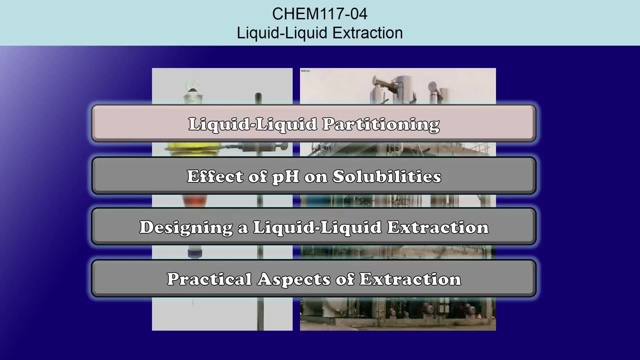 Welcome to the fundamentals lecture for Chem 117, experiment 4.. This week we'll be talking about liquid-liquid extraction. Now, specifically, we're going to talk about liquid-liquid partitioning and what happens when we have two immiscible solvents that are competing to dissolve a 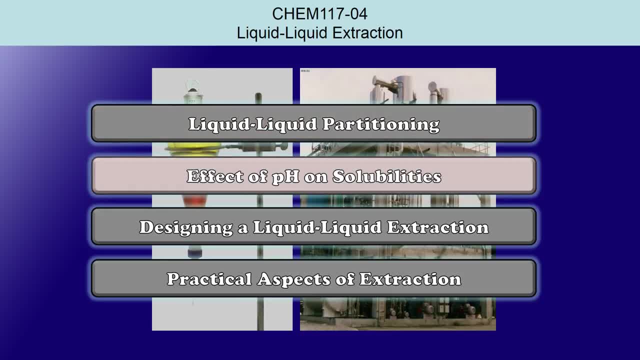 non-volatile organic compound. And once we've figured that out, we're going to ask ourselves: how does the pH of an aqueous layer in one of these systems alter the solubilities and therefore the partitioning coefficients of those compounds? We'll talk a little bit about how we 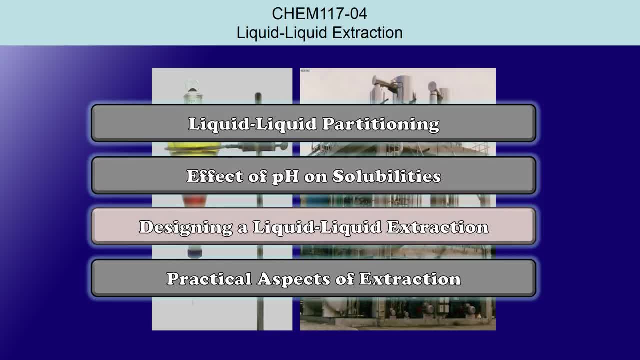 can design liquid-liquid extractions intelligently, knowing how pH affects, or should affect, the solubility of organic compounds in water, And we'll talk a little bit about some practical aspects of how extractions are conducted in the lab and why we use the techniques that we do. 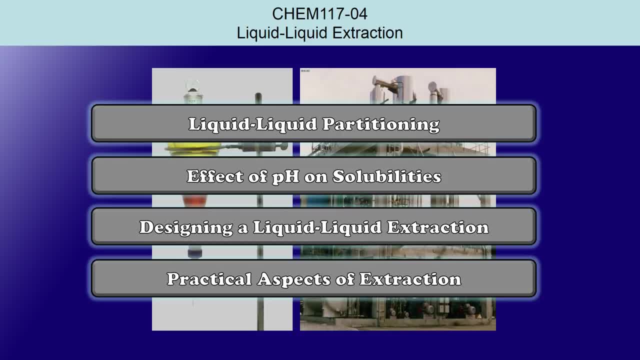 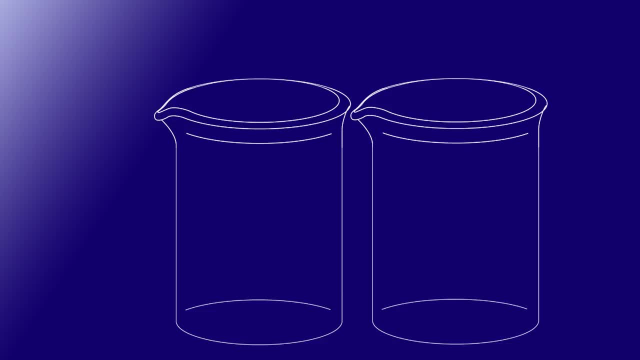 We've got a lot to cover, so let's get started. Let's begin by considering a situation in which we have two immiscible liquids, usually an organic and an aqueous. Now, if I add my water to the beaker here, I get my aqueous phase. 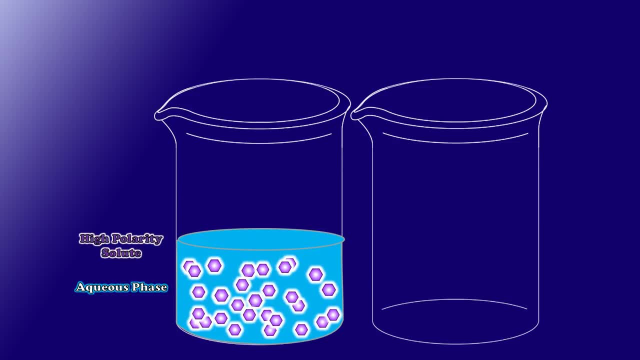 solution. Of course I have to put a solute in there. So let's put in a solute that's very polar, meaning that it makes good strong intermolecular interactions with the water molecules and that aqueous phase. Now I'm going to pour on top of that an organic solvent, something like ether or 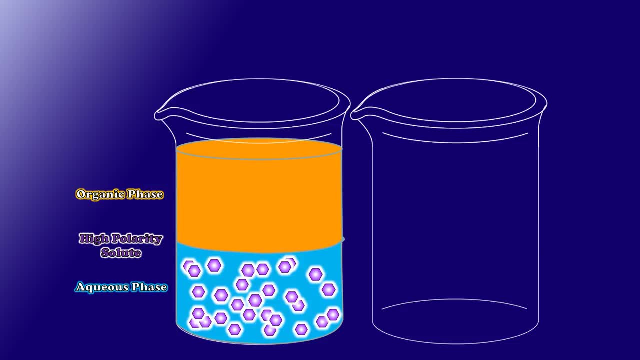 benzene, which will not mix with the aqueous phase because they are what we call immiscible, which is a term that we use in chemistry to describe liquids that don't dissolve into one another. well, Now, what's going to happen when I expose my high-polarity solute and aqueous solution? 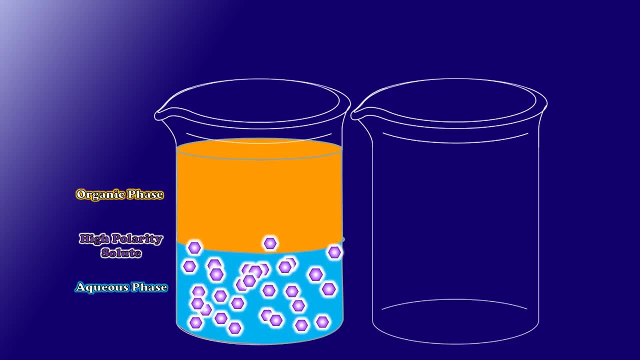 is that a dynamic equilibrium will establish itself in which my high-polarity solute distributes itself across the two phases. But notice that it doesn't distribute itself evenly, that it prefers the aqueous phase more than the organic phase because of its high polarity, and so it has a 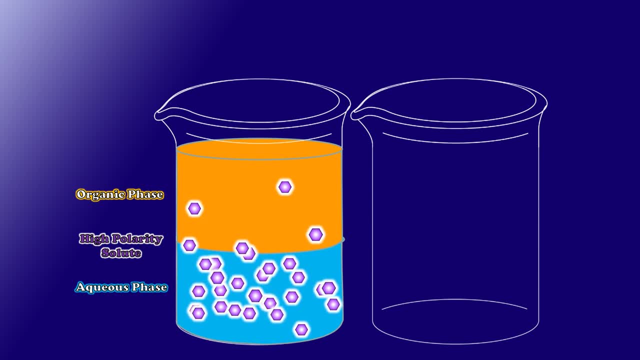 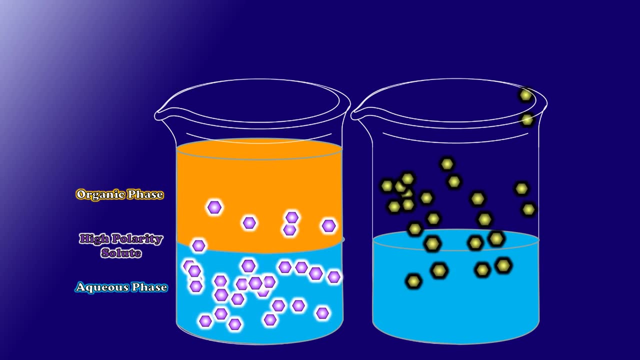 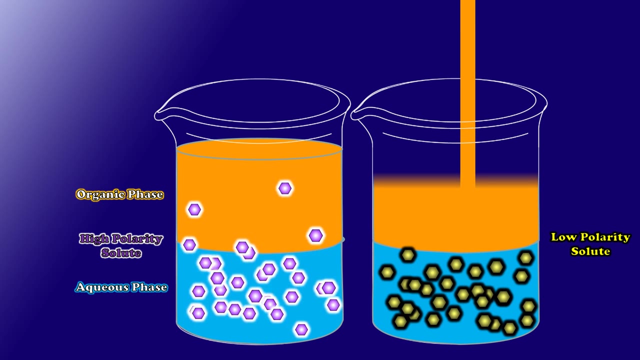 greater residence time in the aqueous phase, meaning it's preferentially accumulated there. Now let's turn our attention to the second beaker. This time I'm going to use an aqueous solution containing a low-polarity solute And again I'm going to add my organic phase to the top here and allow equilibrium to establish. 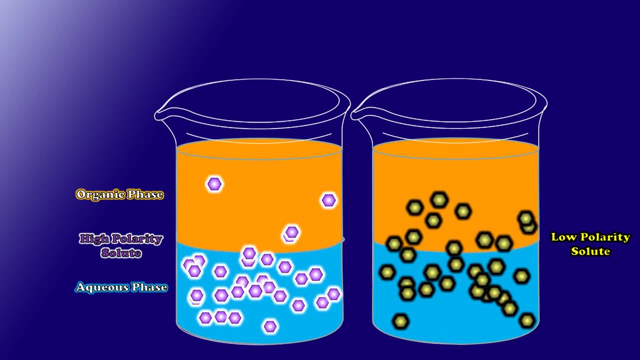 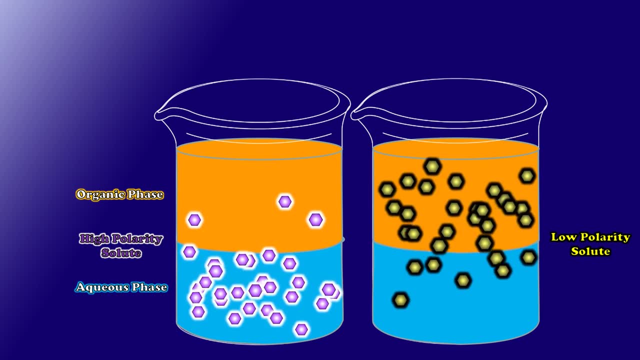 itself, But because my solute in this case is low urban polarity, it has less of an affinity for being dissolved in the aqueous phase and actually prefers the organic phase. So now that the dynamic equilibria are established, we can clearly see a difference here. that 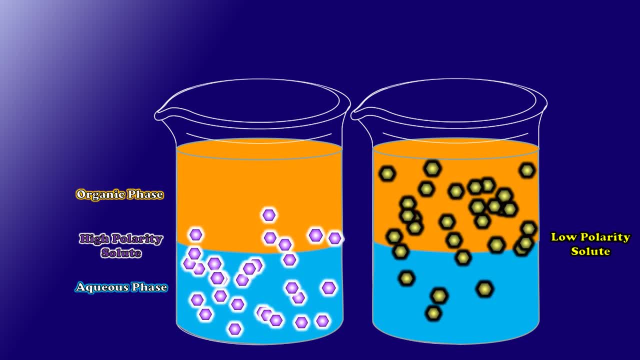 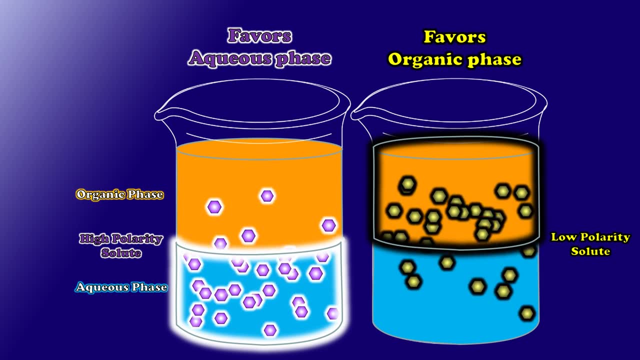 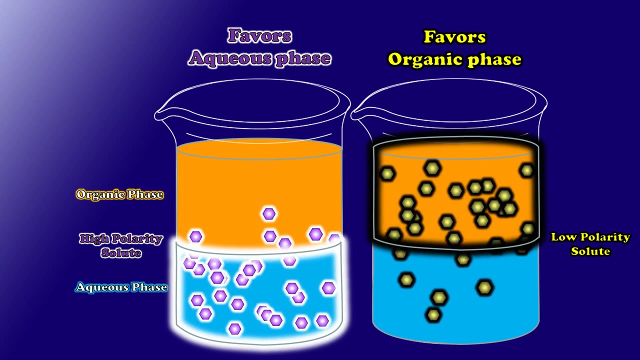 one of my compounds, the high polarity one, has accumulated in the aqueous aqueous phase, while the other has accumulated in the organic phase. This is the phenomenon on which we're going to base our separation technique. We can essentially separate compounds based upon their relative affinities. for one 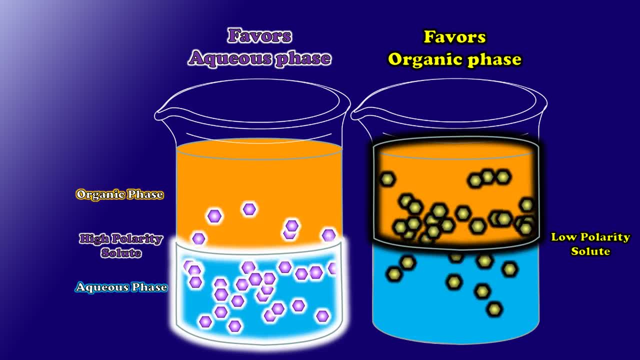 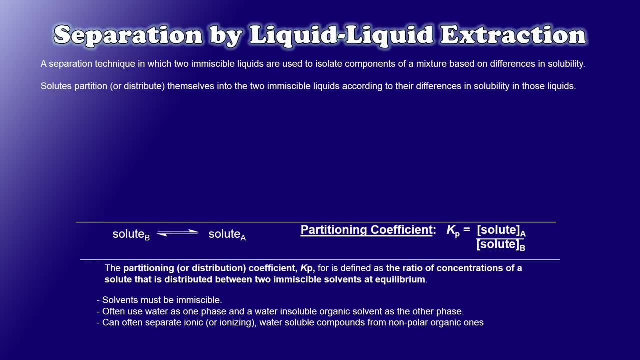 of the two phases. It sounds an awful lot like something we discussed previously, doesn't it? When we use two liquid phases which are immiscible with one another, as opposed to say a solid in a liquid, where one can be stationary and the other. 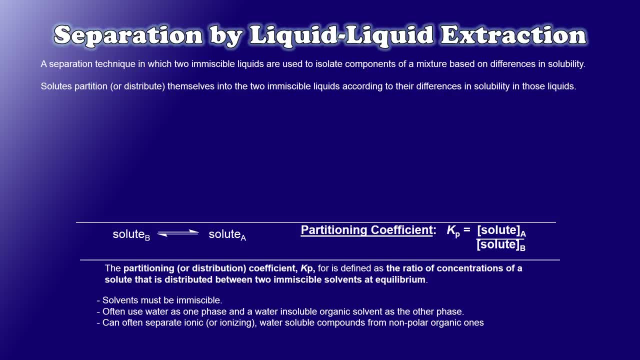 mobile. we use a different name to refer to the technique. We call it a liquid- liquid extraction. It's essentially a technique in which two immiscible liquids are used to isolate compounds from one another based on their solubilities, Because the solvents partition or distribute themselves. 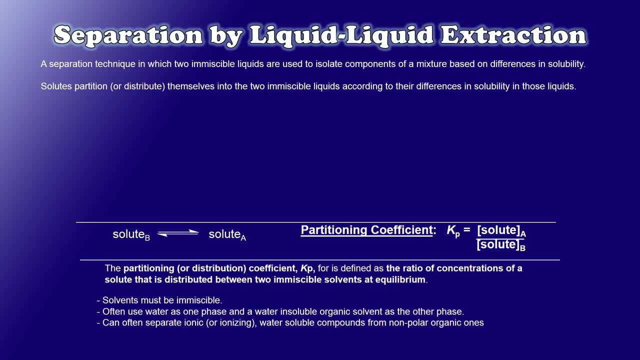 between those phases. we can mathematically model exactly how much accumulates in each layer using an equilibrium constant which we call the partitioning coefficient. So in this case, a partitioning coefficient is simply an equilibrium constant for the concentration in one solute and the 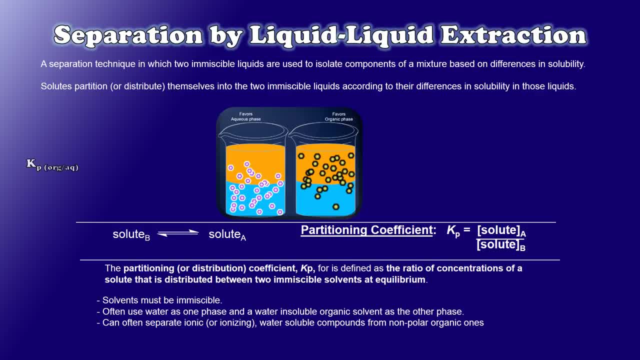 concentration, excuse me, the concentration in one solution and the concentration in another. So on the left hand side, my high polarity compound. if I define Kp or the partitioning coefficient as its concentration in the organic over its concentration in the aqueous phase, I expect that its 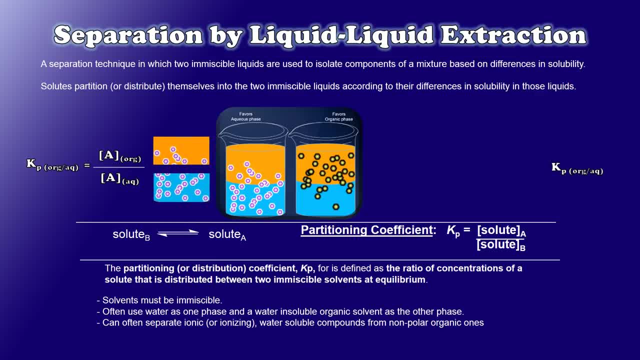 partitioning coefficient will be relatively low because of the denominator is the larger of the two numbers, Whereas in the case of my low polarity compound, if I define Kp as the organic over aqueous, I find that the number is much larger. So what we're looking at here is a situation where 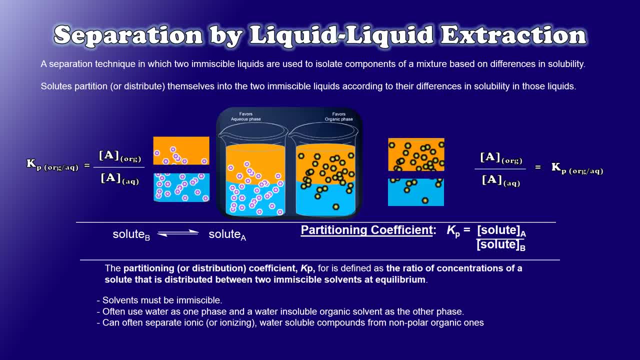 differences in the partitioning coefficient correlate to differences in solubility in the two different immiscible layers. In other words, the more different the partitioning coefficients are, the more easily I can separate one compound from another. That's right. the more different the partitioning coefficients are, the more easily I can separate one compound from another. 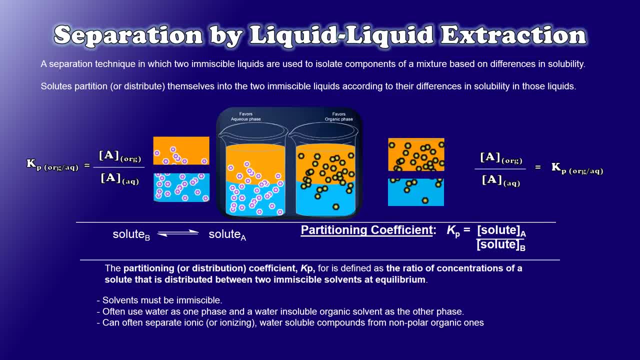 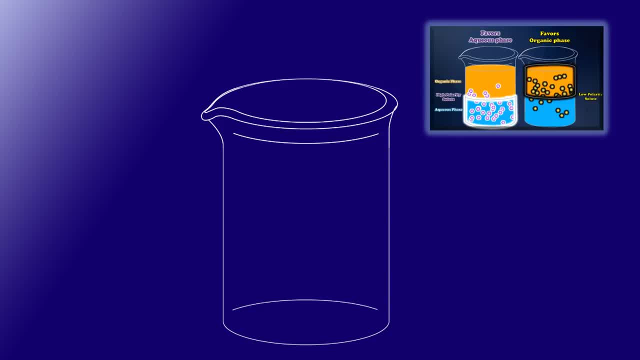 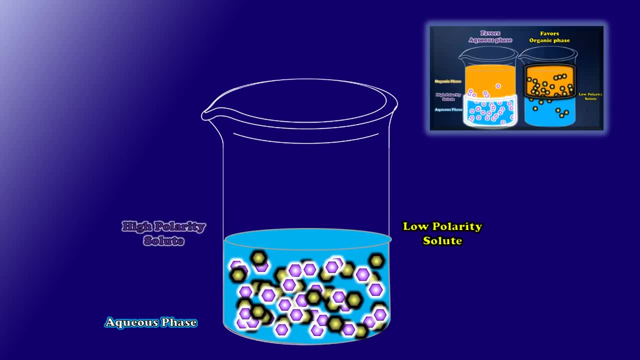 another because they're behaving differently. So if I have a mixture of my low polarity and high polarity compounds and I want to separate them from one another in space, I can take an aqueous phase solution of the two and add an organic phase And, remembering from our previous discussion that they choose to, 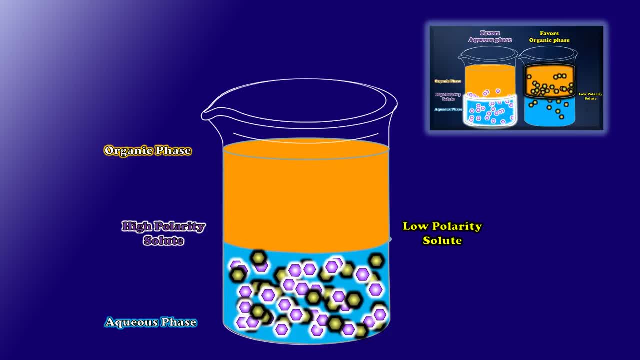 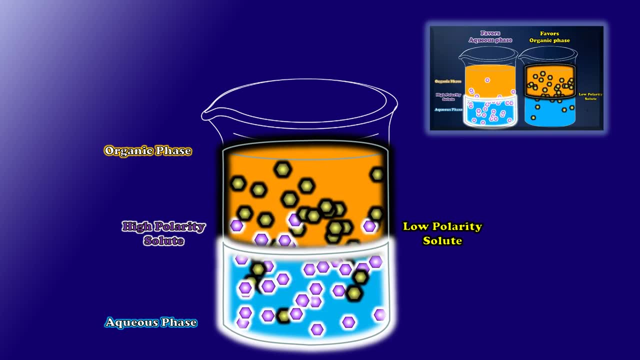 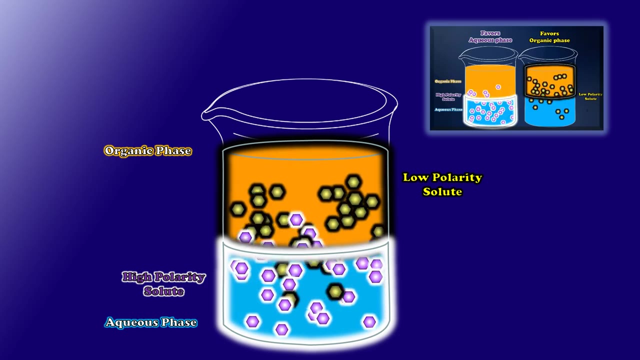 or tend to partition into different layers. in this system, all I have to do is wait for equilibrium to establish itself, And I should reach a situation in which my low polarity solute has partitioned into the organic phase preferentially, and my high polarity solute into the aqueous phase. Now, if I'd 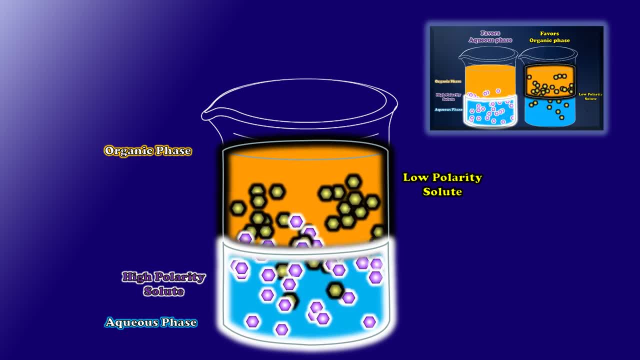 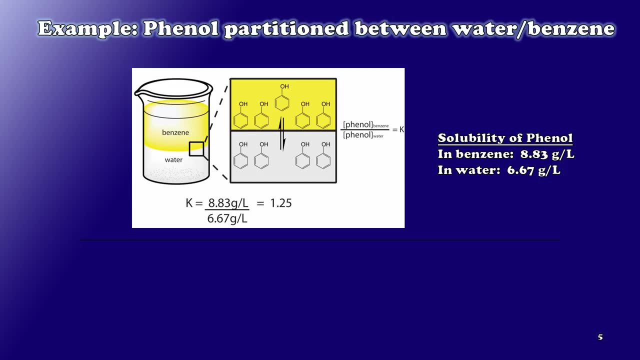 like to collect one or the other. it's as simple as collecting the appropriate phase. Now let's move on from our generic compounds of high polarity and low polarity and start talking about real organic compounds. Let's take the example of phenol And let's talk about how phenol partitions between water and benzene. Now 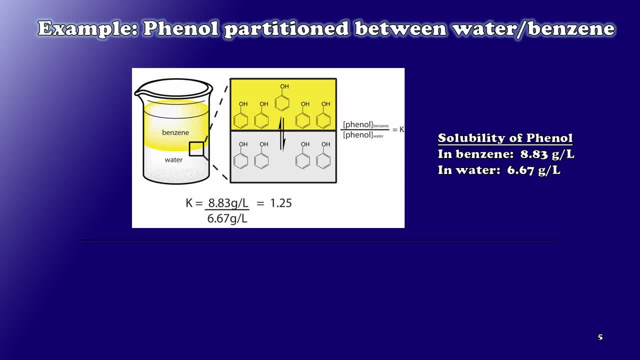 I can determine its partitioning coefficient and I don't have to run a single experiment. All I need to do is go to a data table in a reliable source and locate the maximum solubilities of phenol in the two solvents, In this case. 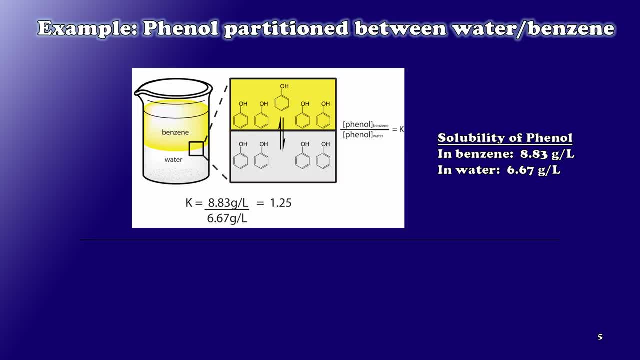 phenol solubility in benzene is 8.83 grams per liter and in water it's 6.67 grams per liter. I can use these numbers to determine whether phenol is a soluble solvent or not, to calculate its partitioning coefficient as 1.25, and I can use that. 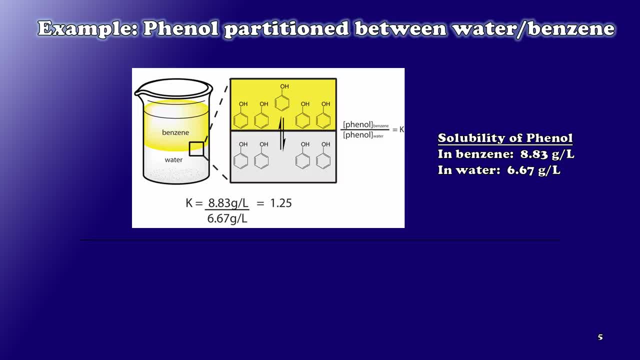 number to predict the outcome or the distribution of phenol in any concentration that I choose. For example, let's suppose we have one gram of phenol dissolved in 250 milliliters of water. I'd like to know if I add an equal. 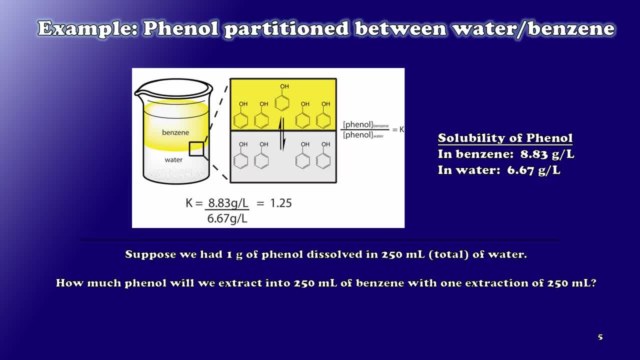 volume of benzene to that and allow equilibrium to establish itself, how much phenol can I expect to be in the benzene layer? Well, knowing that Kp is 1.25 and knowing that the amount which moves out of the water, x grams, must be equal, 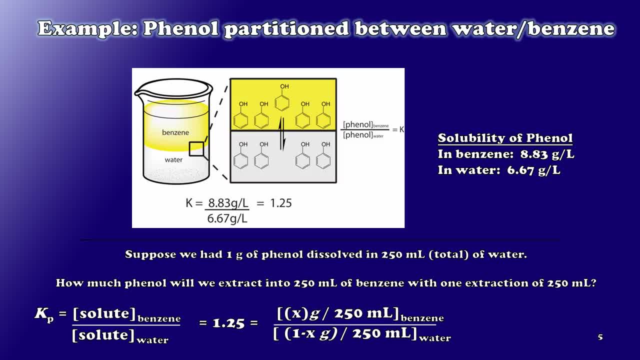 to the amount which accumulates in the benzene. So this gives me a single equation with one unknown, which I can solve using some high school algebra and discover that 0.56 grams of my original 1 gram of phenol has moved into the 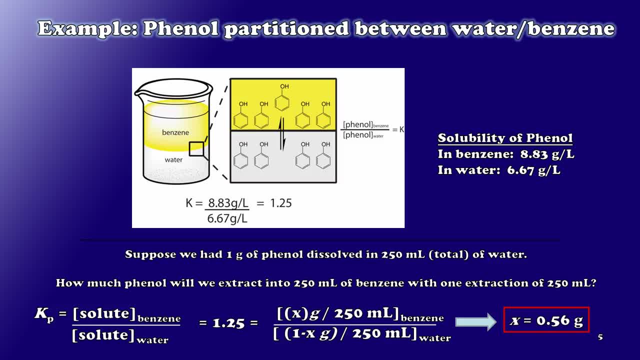 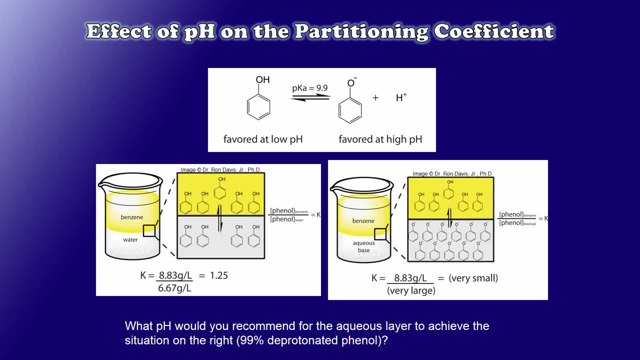 benzene layer. So I can use that equation to calculate the amount of phenol that I need to use the partitioning coefficient to predict where I'm going to find most of my phenol at the end of this process. But is that all there is? Am I at the mercy of this partitioning coefficient? 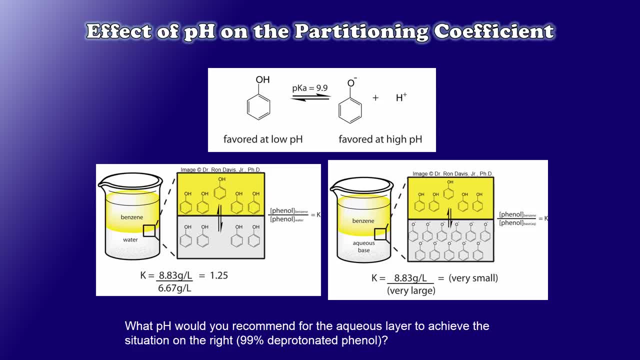 when it comes to moving phenol back and forth between benzene and water? Well, the answer to this question is no. I'm not restricted by that partitioning coefficient, and the reason is phenol is a weak acid and it can be deprotonated in sufficiently basic aqueous solutions. So, while I 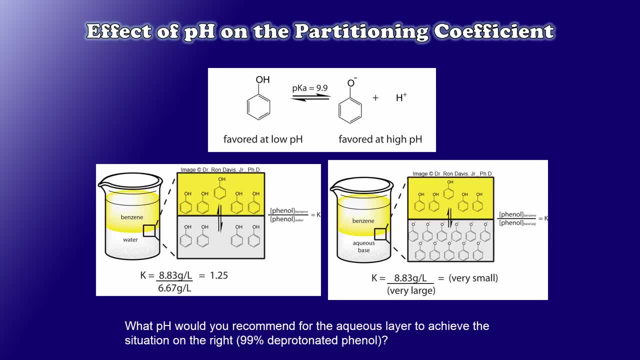 determined my partitioning coefficient to be 1.25 when we're dealing with neutral phenol, as we are on the left side to the slide here. if, instead, I'm using an aqueous base that is sufficiently strong, my equilibrium is no longer neutral phenol in benzene versus neutral. 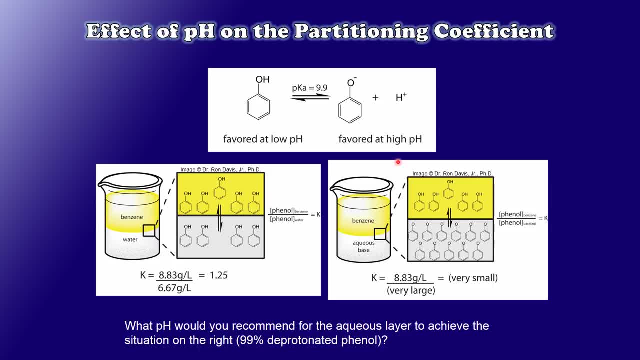 phenol in water. my equilibrium is now neutral phenol in benzene versus charged phenolate, acetic acid anions in the aqueous layer and, as you might imagine, phenolate being charged is far more soluble in water than phenol itself. so i can manipulate the partitioning coefficient. 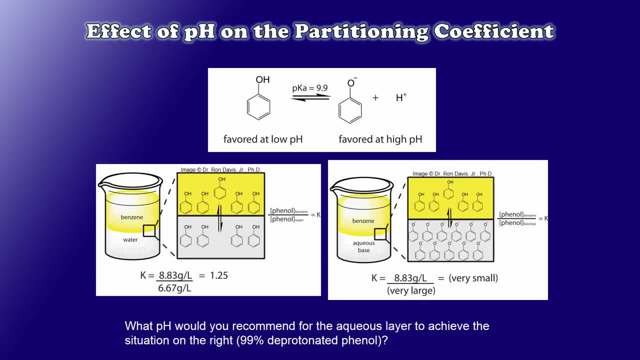 if i make my aqueous layer of the appropriate basic ph in this case. but this begs the question: just how basic does it have to be? let's say i want to get 99 of the dissolved phenol in my aqueous layer to be charged phenolate. this would, within reasonability, maximize its solubility in the 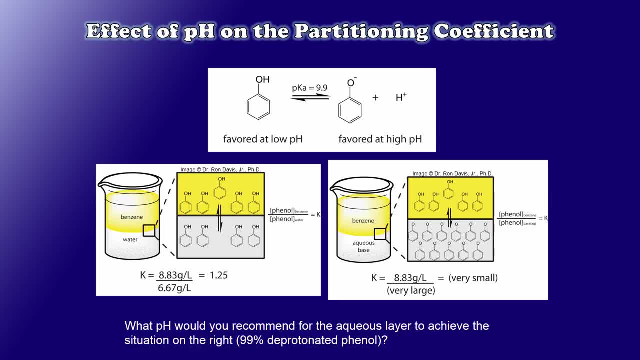 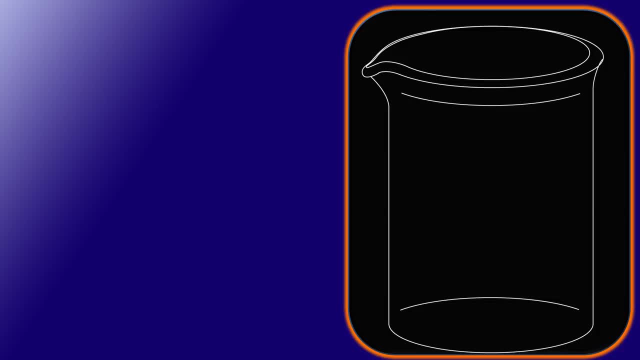 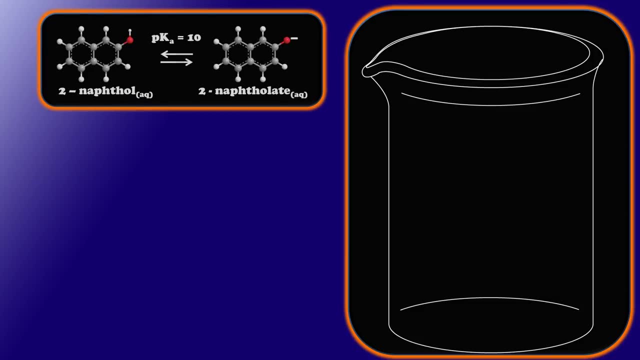 aqueous layer. just how far do i have to go to make that happen? the answer to this question regarding ph and solubility lies in a familiar equation from general chemistry, the henderson-hasselbalch equation. i'm going to demonstrate this using a chemical cousin of phenol known as 2-naphthol. 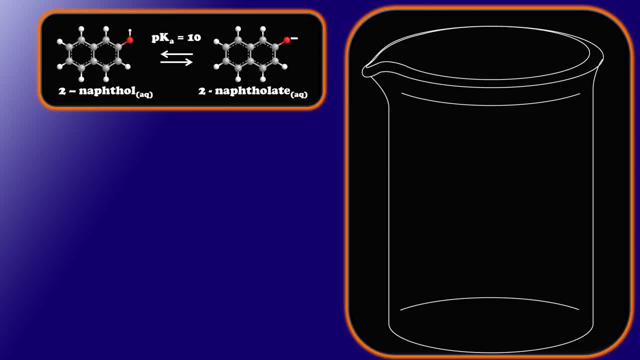 which has fairly similar chemical properties, including a pka of about 10.. the henderson-hasselbalch equation is essentially a rearranged acid dissociation constant which gives me the relationships among the pka of a compound, the ph of the solution in which it's dissolved and the logarithm of the ratio of concentrations. 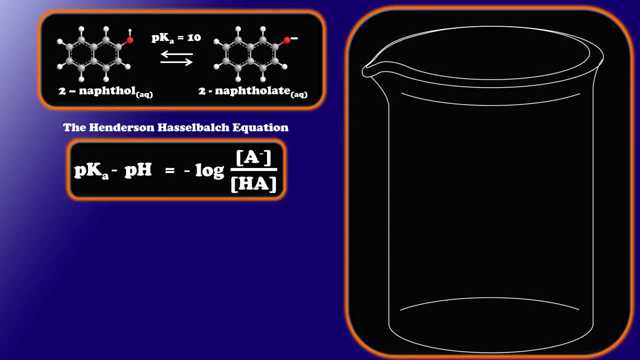 of conjugate acid and base, only one of which, in this case, is ionized. so if i plot the henderson hasselbach plot for 2-naphthol, i get something like this: a situation in which i have 0 percent ionized at low ph, which will be where the conjugate acid is dominant, and 100 ionized at very high ph's. 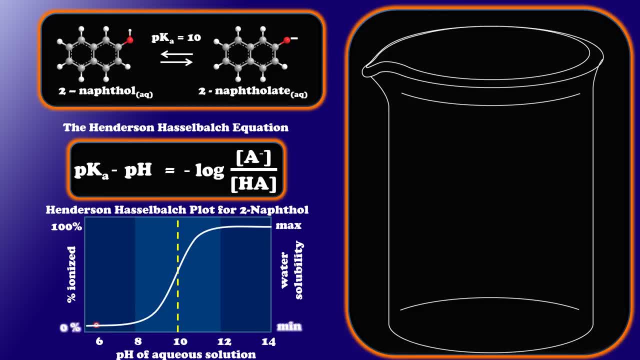 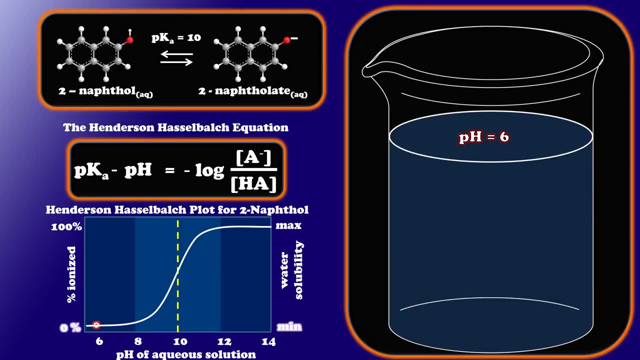 where the conjugate base is what's dissolving in water. now, if i were to take an aqueous solution of about, say, ph6, i can only dissolve a very small amount of naphthol in that because it will be dissolving as neutral naphthol, which is- i've got a little bit polar bond there, but it's. 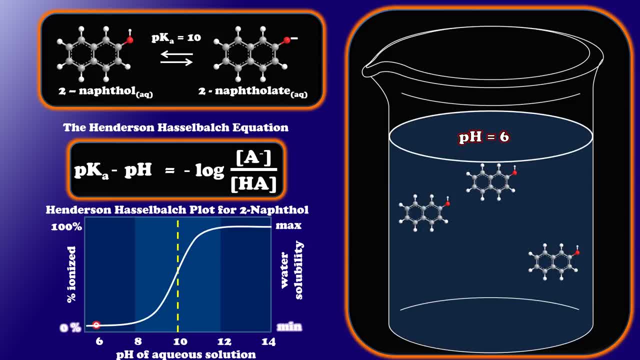 essentially very low polarity and is also uncharged. but if i change the ph of that aqueous layer to something very basic like, let's say, 14. now i'm dealing with not dissolved naphthol but dissolved naphthalate ions, and that means the solubility is drastically increased because the 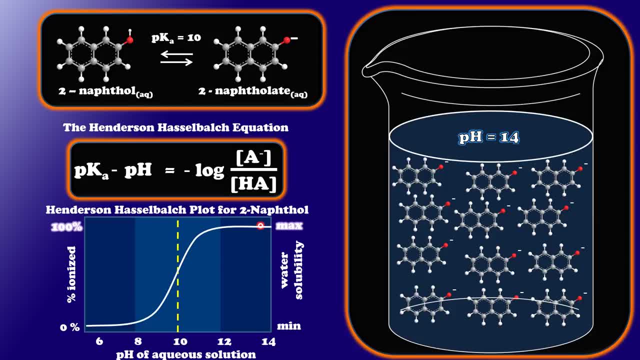 ion-dipole interactions between the naphtholate and the water are much more volatile than the water are much stronger. notice that our relationship tells us from the henderson hasselbach equation that for every unit of ph that we change, we change a tenfold amount of how much. 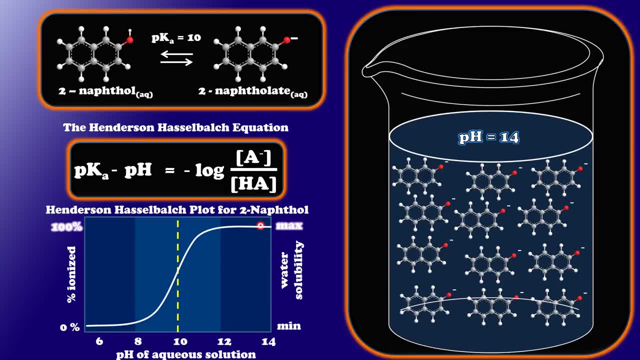 is deprotonated, so it only takes a few ph units above or below the pka of a compound. to maximize this effect and to reach our 99 benchmark we need to go two ph units. so at phs of 12 and beyond we can think of it as being dissolved only as naphtholate and at phs of 8 and below as being. 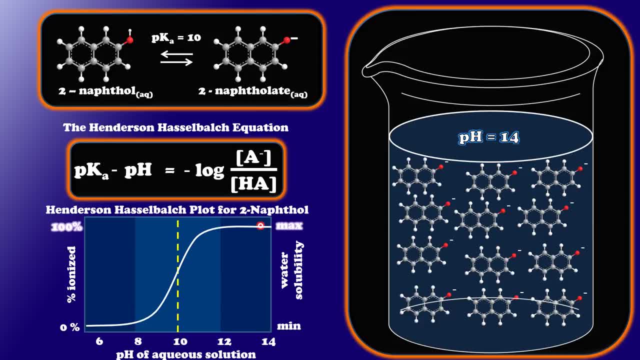 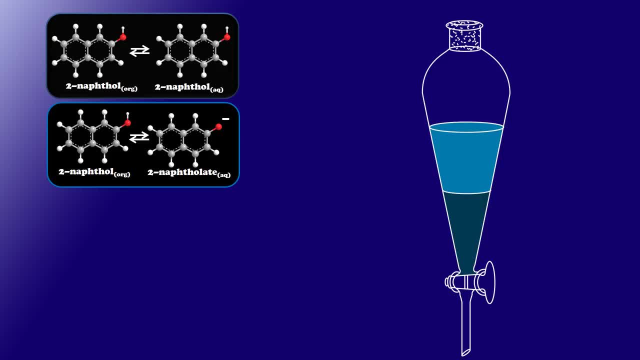 dissolved only as neutral naphthol. so how does this adjusting the ph to alter aqueous solubility impact the outcome of liquid-liquid extractions? let's begin by thinking just about naphthol, but this time, instead of in only water, it now has a second phase that it can partition into in the 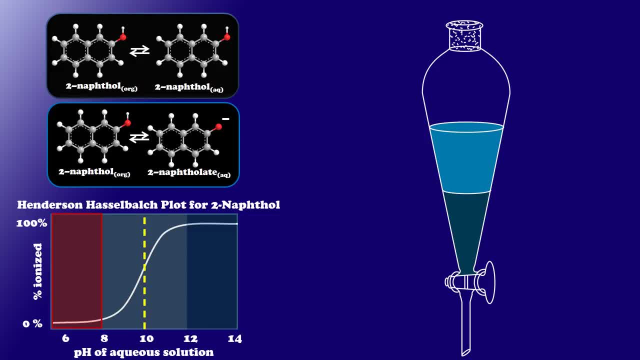 organic. remember my henderson hasselbach plot tells me that at phs of 8 and below, i'm dealing with naphthol dissolved in water, but at phs of 12 and above i'm dealing with naphtholate. now let's take a look at what goes on in this interface between our two solvents. 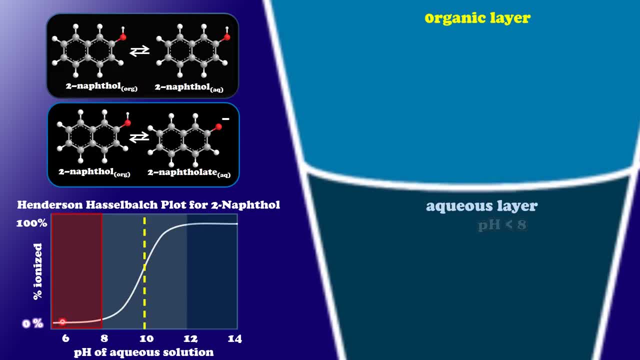 as we change the aqueous layer, ph. at ph is less than 8, we have a situation where the equilibrium is that between neutral naphthol in the organic and neutral naphthol in the organic and neutral naphthol in the organic. 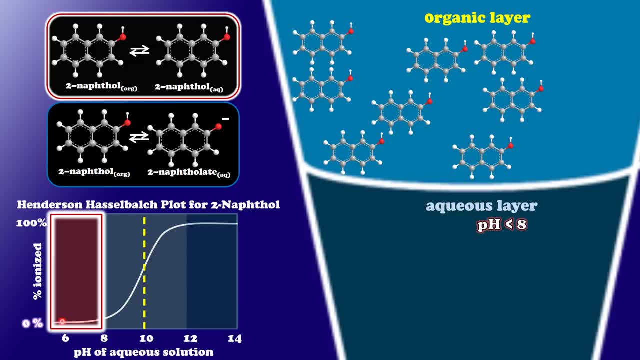 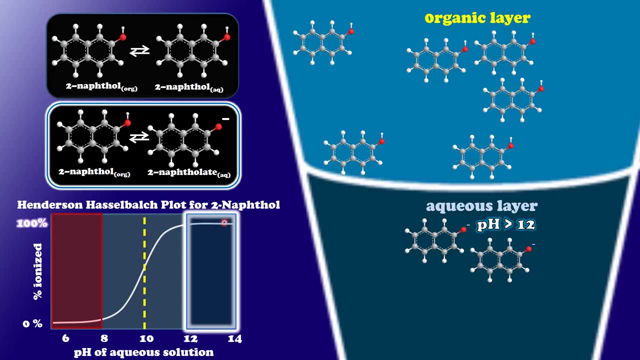 and neutral naphthol in the water, meaning that it's going to prefer to be in the organic phase and only a small amount will dissolve into the water. but as i change the ph of the aqueous layer again moving up to something like 12, 13 or 14.. now i'm dealing with dissolved naphtholate. 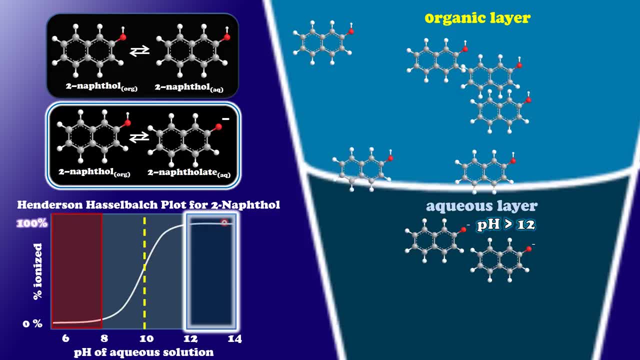 whose concentration is much greater and therefore i expect more of the naphthol to partition into the aqueous layer so i can alter the ph of my aqueous layer as shown in this slide, where the intersection raid of smooth doesn't exist. now we've that new. 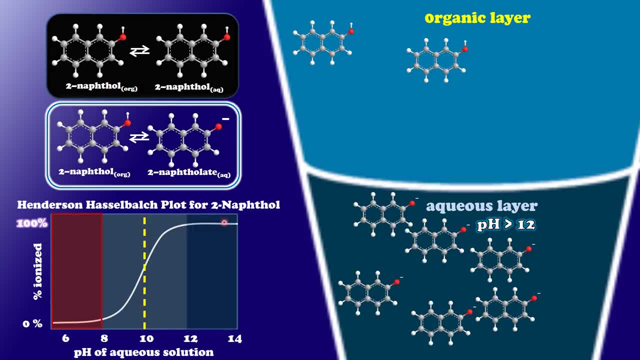 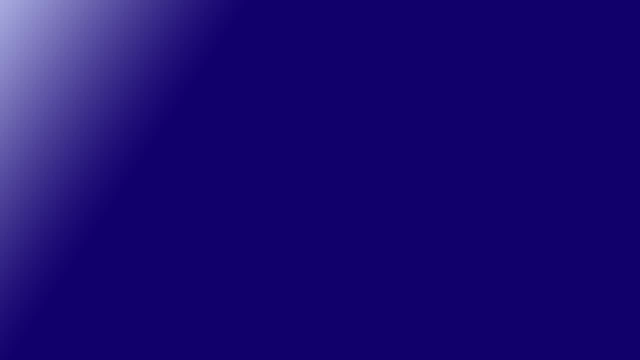 phase for this시간 of Voyager io. two, three, three seconds gain over here because, as we have seen, when we use this one phase, the need for this naphthol to distance itself is much greater. as we go about to take a look at ourument to thisnext phase of the aqueous layer ph. 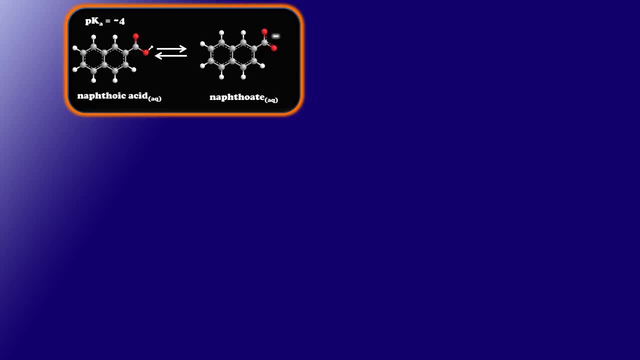 so what we can do, if we're actually looking at this phase of the aqueous layer ph, is by connecting ourde крes aqueous layer ph with the higher one phase of the aqueous layer. ph has a pKa of about four as opposed to 10.. 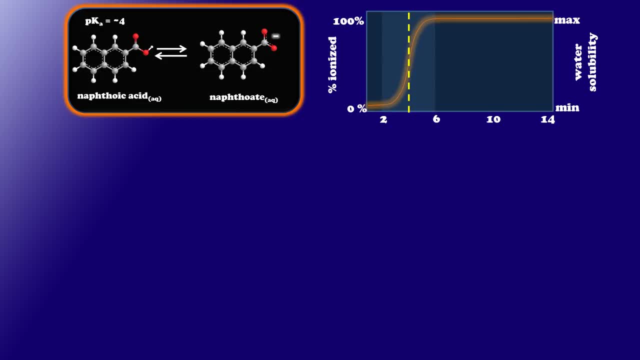 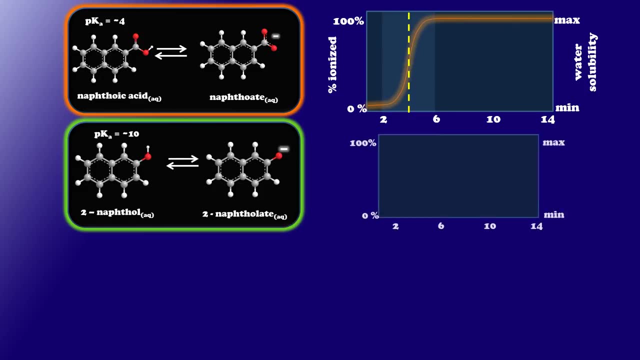 So it's Henderson-Hasselbalch plot will look something like this, with its break point at around pH four. We've already seen how nathol will have a Henderson-Hasselbalch plot which has a breaking point somewhere around 10.. 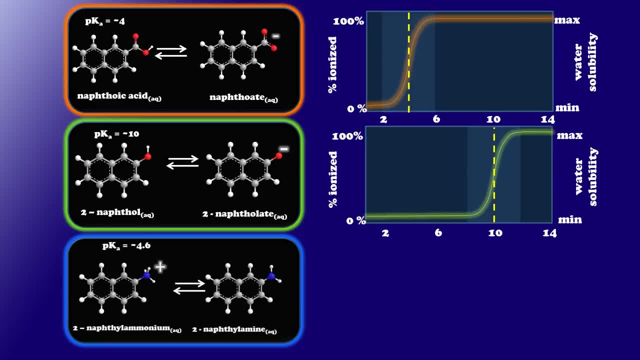 A third compound to consider in a different situation would be a compound like naphthalamine. Now notice that naphthalamine is actually a base, so it's charged at lower pHs as opposed to at higher pHs. So its Henderson-Hasselbalch plot. 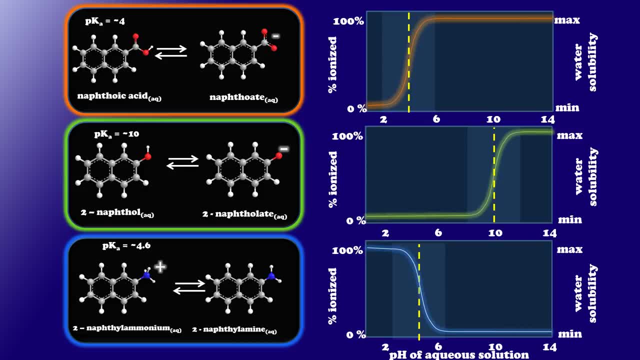 will be turned on its head, as it were, with the greatest percent ionized at lower pHs, And its break point is determined by the pKa of naphthalammonium, which is about 4.6.. So how can I use these Henderson-Hasselbalch plots? 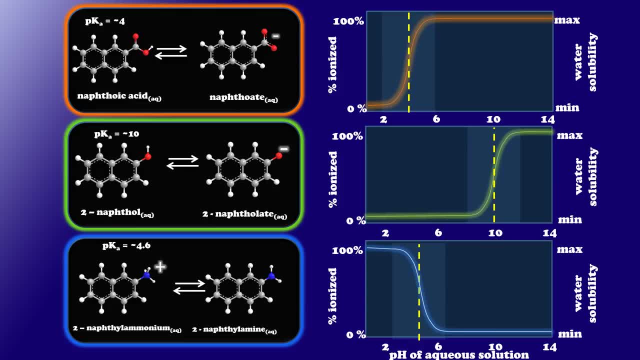 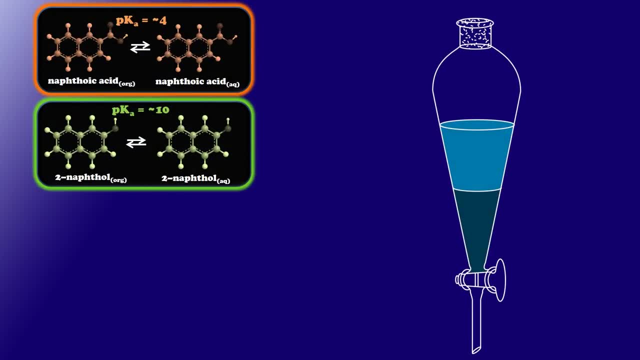 to graphically guide my decision on aqueous layer pHs to optimize extractions, Let's first look at our 2-week acids. We can calculate the pH of the two acids from aqueous to liquid. Now let's consider our 2-week acids. 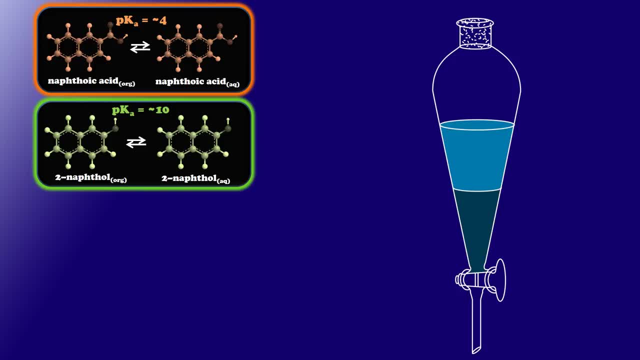 and how we can separate them, or at least design a separation using liquid-liquid extraction. Let's say we have two different phases in a separatory funnel, the device pictured on the right here. We'll talk a little bit more about the device itself later. 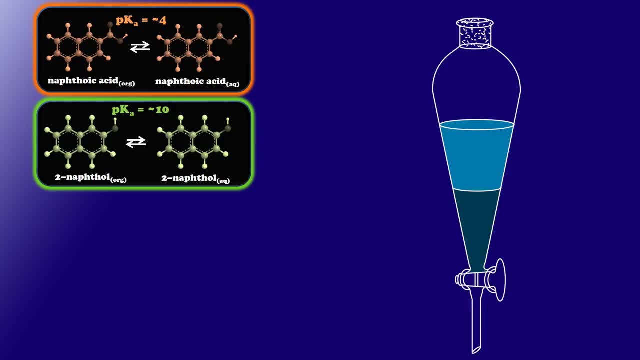 What we're interested in right now is, depending upon the pH of the aqueous layer, what goes on at this interface between the two? Where are we going to find the pKa, going to find most of these compounds? Well, we can overlay their Henderson-Hasselbalch plots. 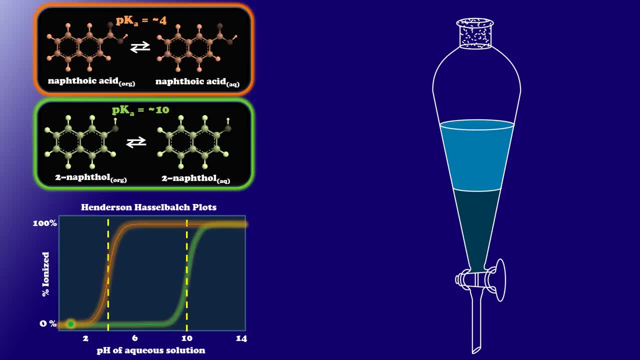 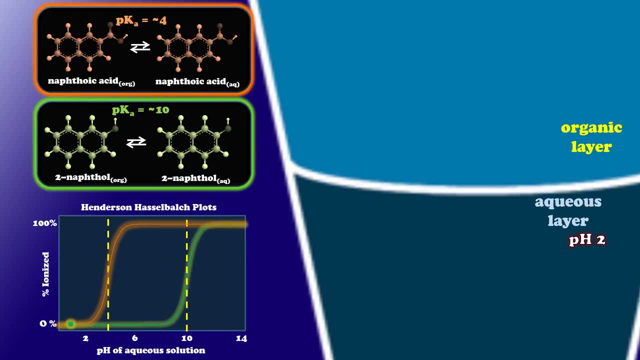 and immediately see that there are some similarities and some differences. Let's begin at a very low pH. Let's say that I have an organic layer above an aqueous layer with a pH of 2.. This puts me down here in the Henderson-Hasselbalch plot, in a region where 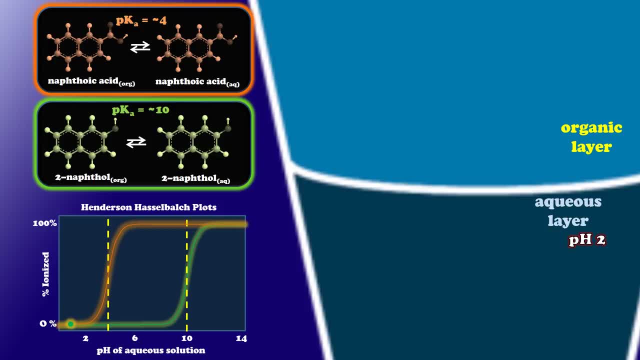 neither one of them is substantially ionized when they're in the aqueous layer, So I expect them to preferentially accumulate in the organic layer, because we're dealing with the solubilities of these neutral compounds and they don't like to go into water when they're. 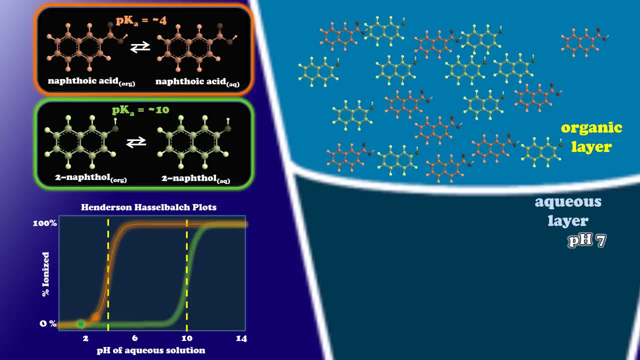 neutral, But if I change that pH to 7, there's a huge difference between their percentage of ionized, meaning that I expect my naphthoic acid to move into the aqueous layer as naphthoate anion. 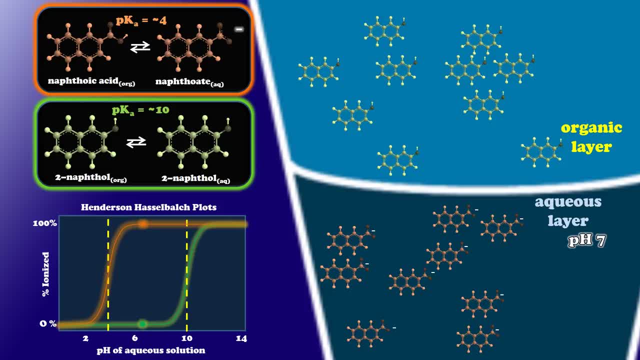 At this point. if I were to separate my two immiscible phases, I would have to separate my two immiscible phases from the aqueous layer. I would be affecting a separation of the two compounds. But if I continue and raise the pH even higher in the aqueous layer, let's say that I go to pH 12,. 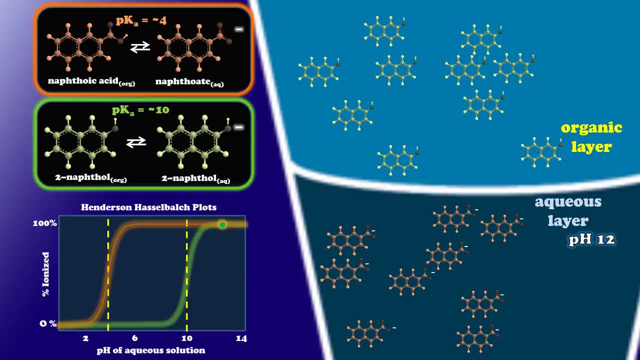 now I'm in a situation where both compounds dissolve in water as ions and that means that the naphthol is also very soluble in water and therefore will partition into that layer. So separating my phases at this pH also would not affect the separation of my compounds. So the key here is to separate the two compounds from the aqueous layer. If I continue and raise the pH even higher in the aqueous layer, I would be affecting my two compounds as naphthol. So the key here is to separate my phases. at this pH also would not affect the separation of my compounds. 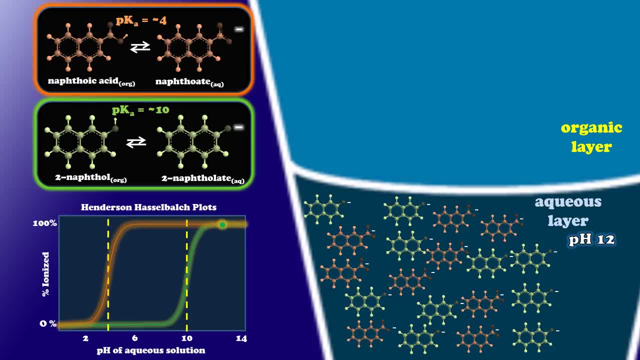 So the key here is to separate my phases at this. pH also would not affect the separation of my compounds- The greatest difference in the Henderson-Hasselbalch plots for your two compounds and use that as the pH of your aqueous phase in order to direct one compound into the water and keep another one in the organic. 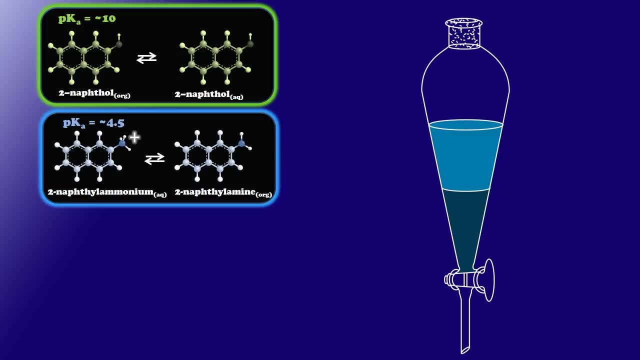 Now let's take a look at what happens when we're dealing with acids and bases. Remember that naphthalammonium and naphthalamine are a bit different, because in this case we have the charged species in the lower pH, in the baryonyl and in the aqueous. So the pH of the baryonyl and 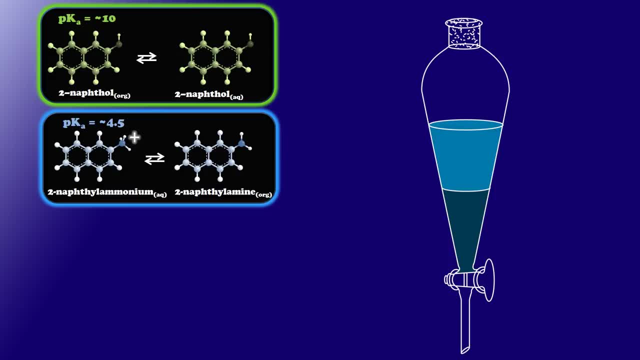 species in the lower pH region of our plot. So the Henderson-Hasselbalch plots for these two compounds look something like this, So you can see what's going on here. Now, as opposed to having the greatest difference at moderate pHs, we 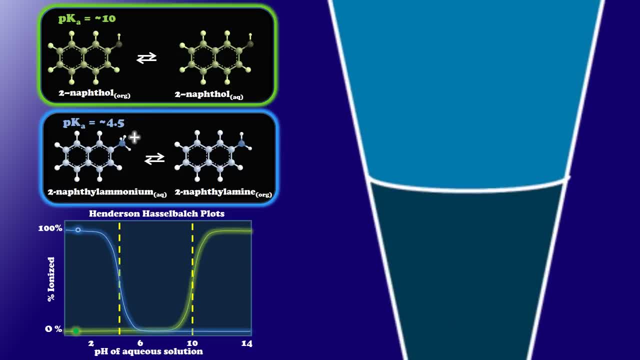 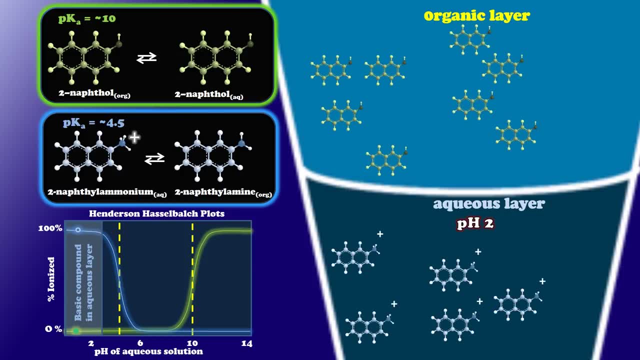 get a very large difference in the percent ionized at low pH. In this case that's going to favor our basic compound, the naphthalamine, accumulating in the aqueous layer. But if we raise that pH to 7, which worked great for us last time- 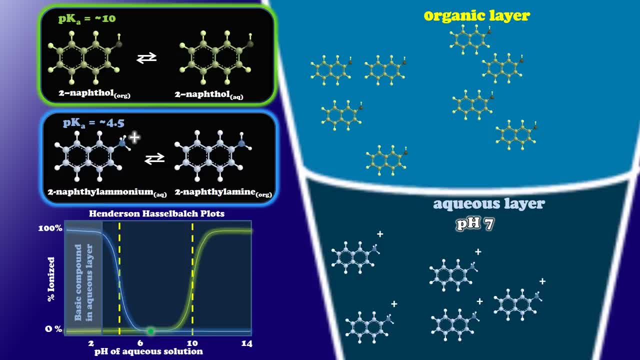 we run into a problem because now they have very similar water solubilities and that means we're not going to have a very good separation. In this case, both of them will accumulate in the organic layer more because they're not charged. 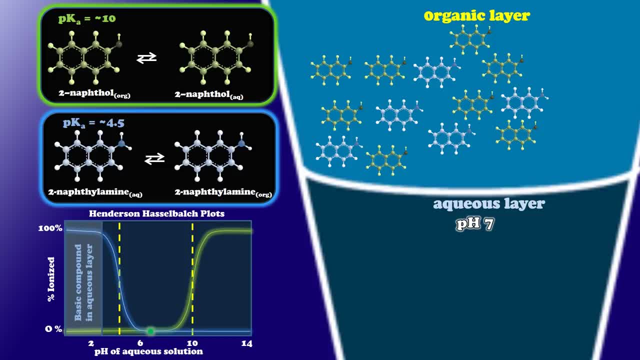 when they're dissolved in water. at this pH, Continuing on further to another extreme, at very high pHs, my naphthol is expected to migrate to the lower pHs. So we're going to have a very large difference in the aqueous layer because it's dissolved as naphthalate. So we can see here one 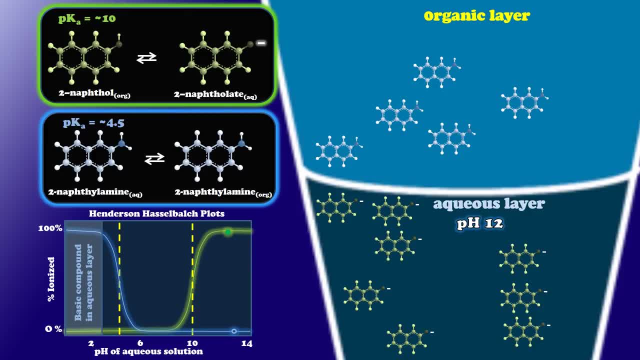 benefit and one drawback to separating organic acids and bases, The benefit being that we get to pick which layer each one moves into, but the drawback being that we have to use very strong acids and bases to accomplish it. Now it's time to talk a little bit about the practical aspects. 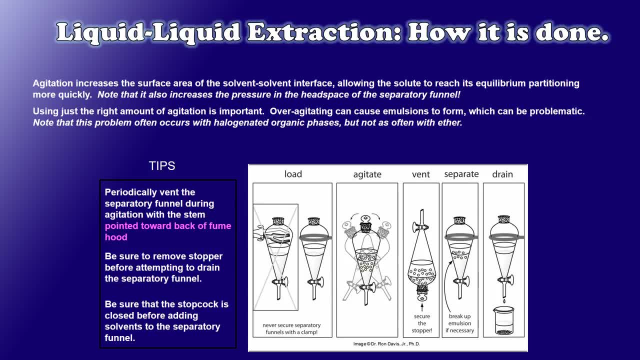 of liquid-liquid extraction. We accomplish liquid-liquid extractions using a device known as a separatory funnel, which is this gadget down here, which is sort of a conical shaped device with a Teflon stopcock at the base and an opening at the top through which we can add different solvents and different 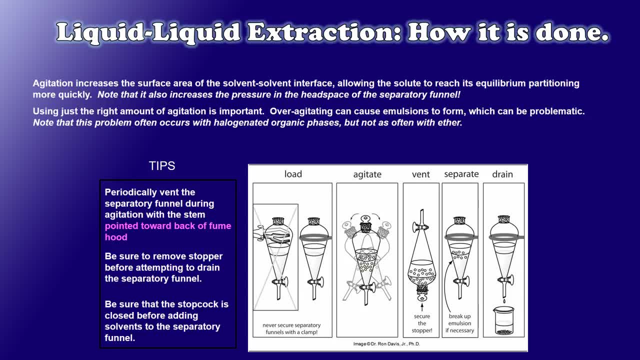 compounds. The first thing I want to point out here is that we never clamp one of these devices using two or three fingered clamps. They're simply not stable enough. Instead, we use a metal ring clamped to the rail that's just a little bit narrower than the top of the flask, So when it's 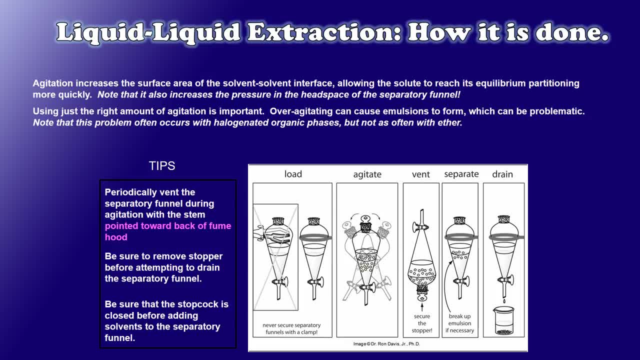 inserted and lowered downward, it eventually stops and is held in place by that ring. Now to begin the process of conducting a liquid-liquid extraction. we load a solution into a separatory funnel supported by a ring. We simply pour our solutions and solvents in through the top, being sure that, of course, the 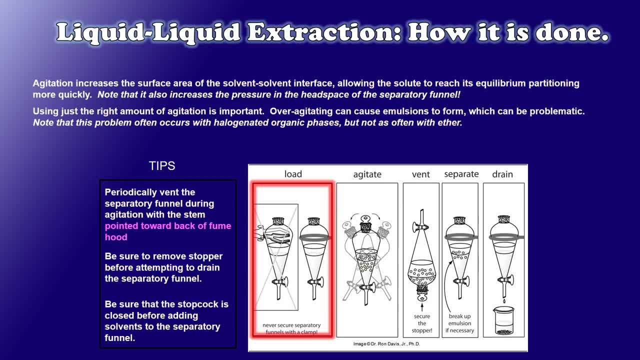 stopcock at the base is closed at the time, so that everything stays inside. The next step is to agitate. We agitate to speed up the rate at which the equilibrium is established, to be sure that we get the proper distribution of compounds across the two phases, And this is done by placing a stopper in the 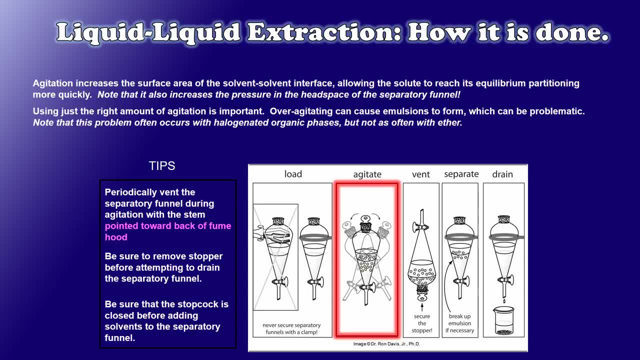 opening of the separatory funnel and then inverting it back and forth several times over the course of a minute or two. Periodically, we want to be sure that we vent our separatory funnel to prevent pressure building up from either solvent vapors or byproducts of the process of the partitioning. This is 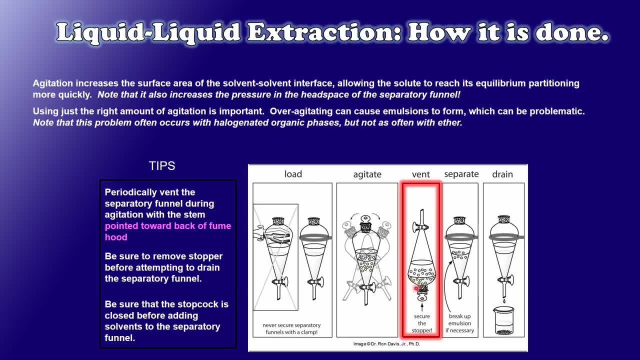 done by inverting the separatory funnel, being sure that you hold the stopper in place with your finger, and then, with the top vent pointed back into the fume hood, we open the stopcock and this releases the pressure. The stopcock is. 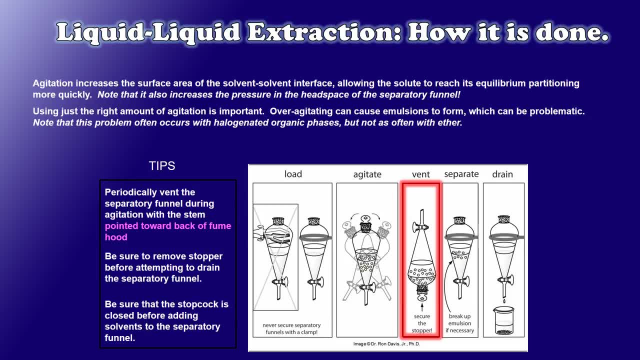 then closed and agitation can continue. Once we're confident that equilibrium has been reached, we allow those two phases to separate once again by returning the separatory funnel to the iron ring and allowing gravity to cause our two immiscible phases to separate based on their densities. Occasionally, we get what's known as an emulsion, which 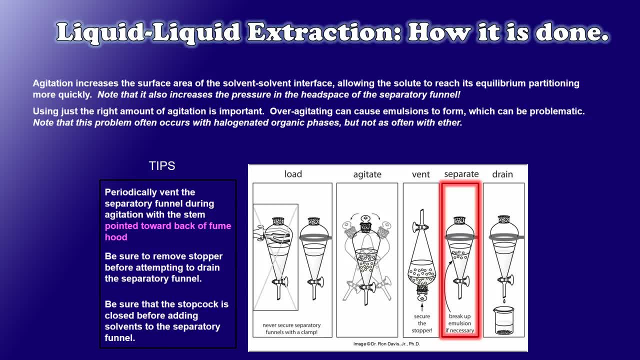 is where very small droplets of one solvent and the other become sort of metastable and don't really want to separate. well, And when this happens we can usually break up an emulsion by very gentle agitation with a glass stir rod. Once the phases have completely separated, we isolate them from one. 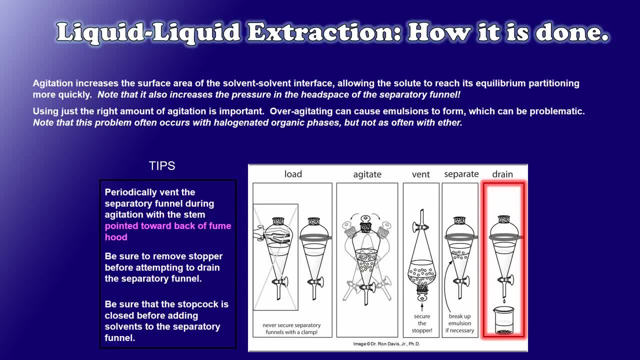 another in space by opening the stopcock, being absolutely sure that the stopper is removed and then allowing the lower of the two phases to drain out of the separatory funnel into a collection flask or beaker. At this point we should have physically separated our compounds in space using liquid-liquid extraction. 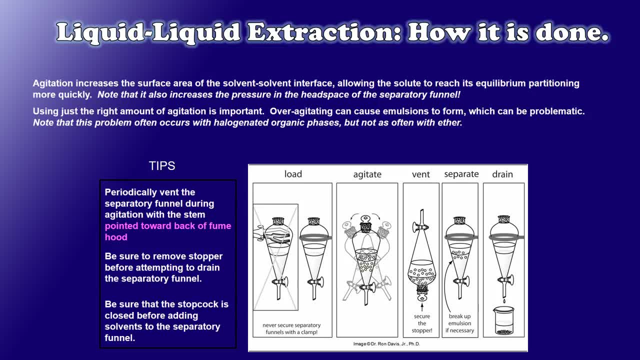 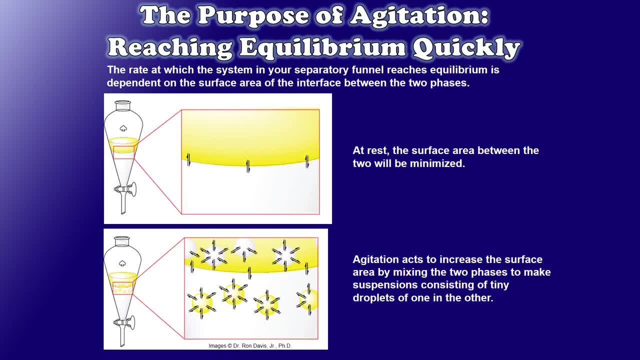 So why do we go to the trouble of agitating during an extraction process And why is it so important that we do it? The reason is this: We want to reach equilibrium as quickly as possible. We're relying on equilibrium constants to predict the outcome of an extraction, so we have to be sure the system really is. 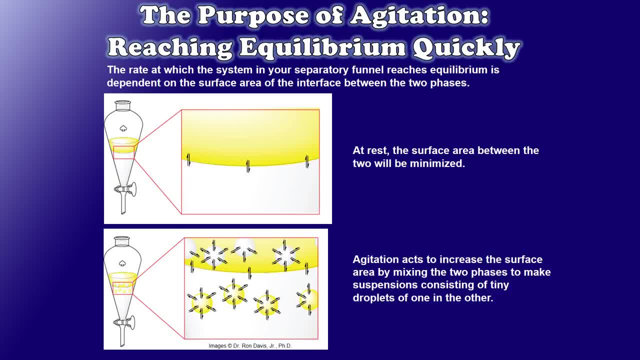 at equilibrium before we begin separating one layer from the other. Now imagine two different immiscible liquids in a separatory funnel. at rest, The only surface area contact is that very thin interface between the two solvents. So in order for a compound to migrate from one to the other, it has to 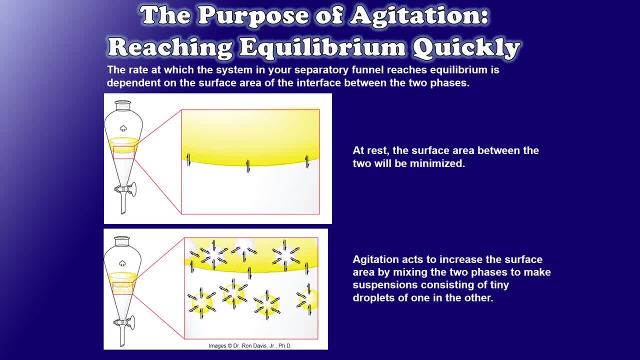 find its way to that interface and with a bunch of molecules taking random walks through the solution, this can take a very, very long time. But by agitating sufficiently we create small inclusions of one solvent in the other, And this means that there's a tremendous amount of surface area contact. so 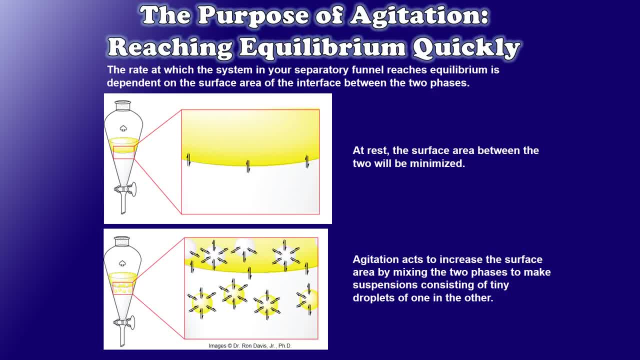 molecules have much greater opportunity to partition from one phase to the other, thereby reaching the equilibrium much faster. So when we do agitation, you want to be sure that you're creating these small inclusions of one solvent in the other. If agitation is too gentle, it won't accomplish anything. If agitation 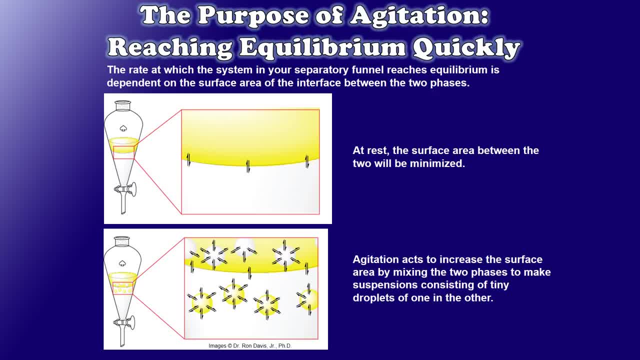 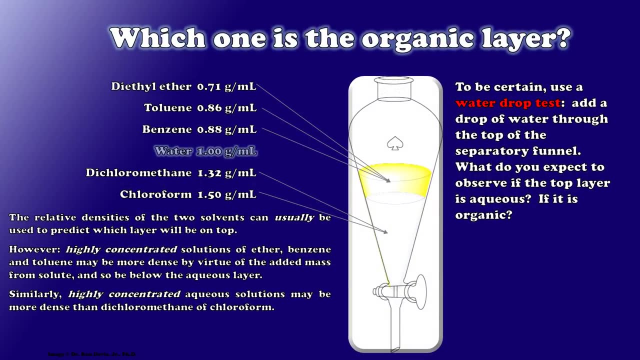 is too vigorous, you run the risk of creating an emulsion. So getting just the right amount of agitation is actually a very important skill to hone to be sure that your liquid-liquid extractions always turn out the way you expect. So another logical question comes up here If I'm creating these. 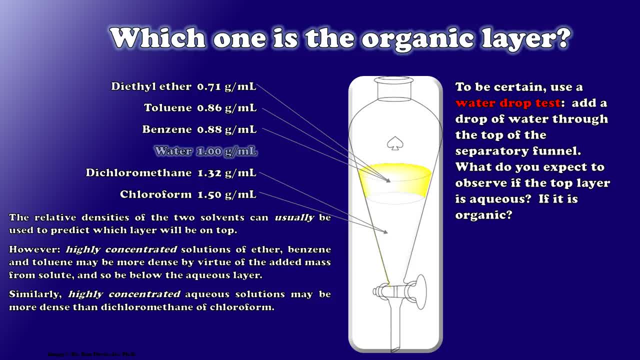 inclusions of one solvent in the other and really shaking things up during the agitation process. how do I know which solvent is the one on top and which is the one on the bottom after I'm done and the phase separation process begins? Now the answer is we use something called a water drop test to be 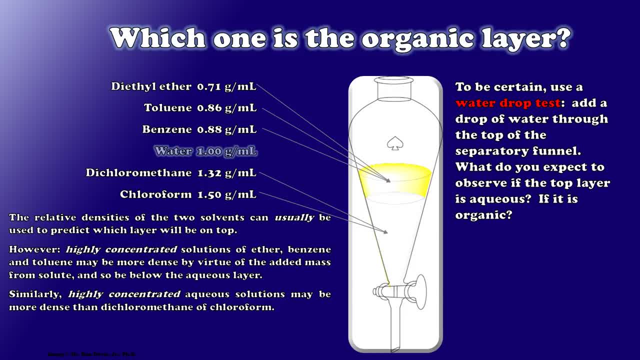 absolutely sure. Typically non-halogenated solvents like diethyl ether, toluene and benzene can be expected to be the top layer in a liquid-liquid extraction, because their densities are less than that of water. Halogenated solvents on. 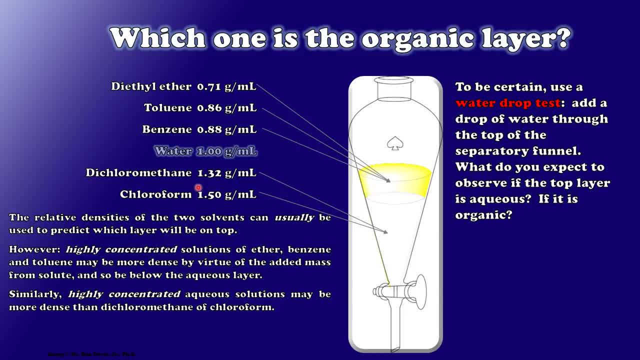 the other hand, like dichloromethane and chloroform, have densities that are substantially greater than that of water and therefore where they usually accumulate an emulsion As the lower layer. But there's a catch there We're dealing with here with the 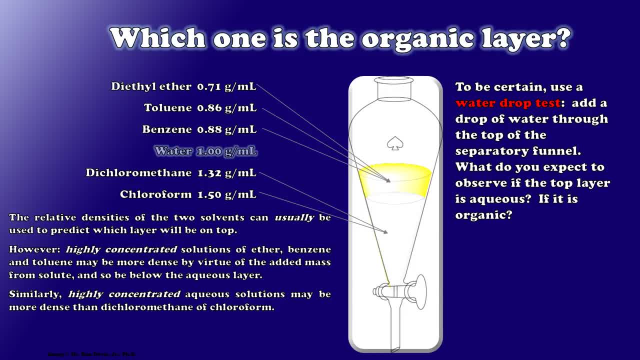 densities of solvents, but what really dictates the behavior is the density of the solution, And a solution with a large amount of very high mass solute might defy prediction here. So we need a test that will absolutely let us know which layer is which. For this we use what's called a water drop test, in which we 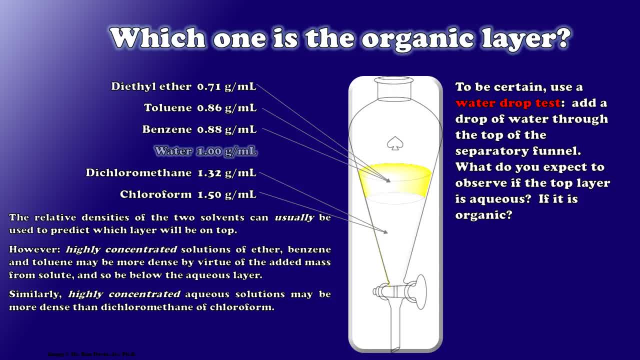 add a drop of water through the top of the separatory funnel And, depending upon what we observe, we will know whether that top layer is aqueous or organic, because water should mix well with aqueous solutions but not well at all with organic solutions. So think about what you expect to observe in different. 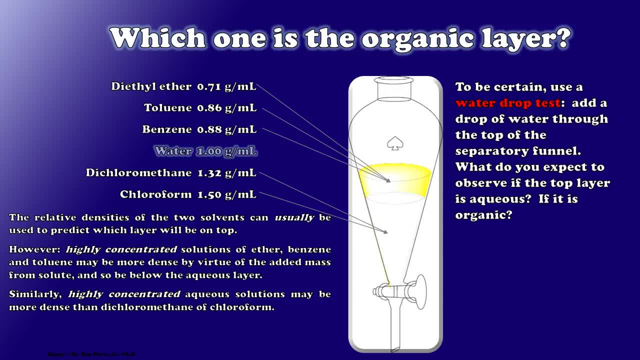 situations and be ready to discuss that when you come for recitation. This is a big gotcha in the lab. You've got to know which layer is which, because if you don't, you may end up collecting the wrong layer and throwing your compound. 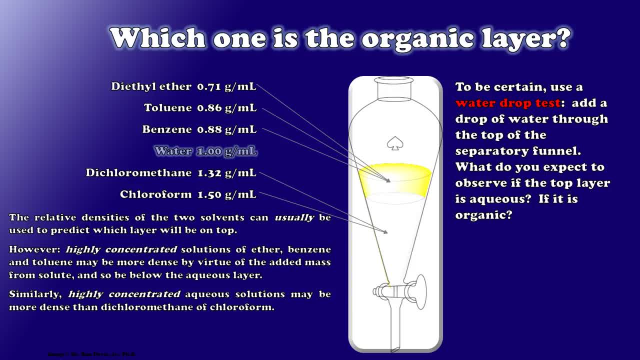 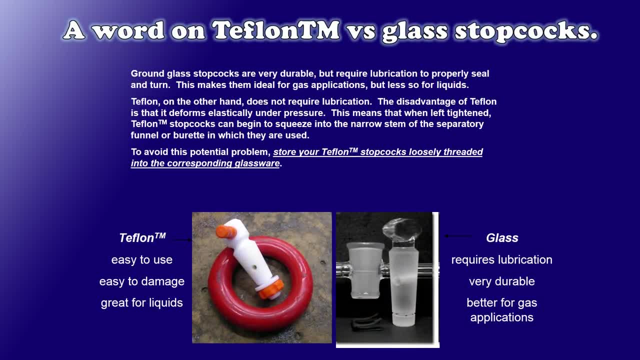 into the chemical waste, So water drop test every time to be sure. I'd also like to mention that the stopcocks that are used in our separatory funnels are made of Teflon, which is a fantastic material for liquid applications because it. 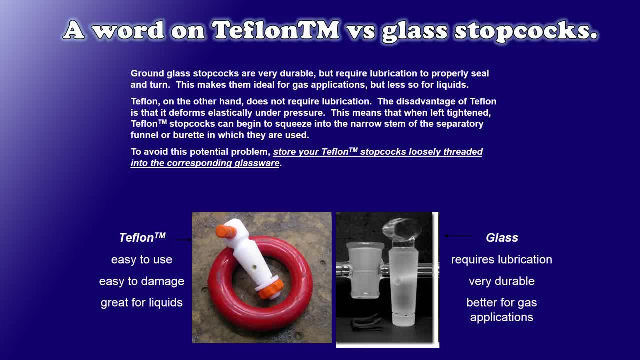 requires no lubrication. So when we use a Teflon stopcock, we don't have to add grease to a joint, and that means that liquids draining through and over the stopcock don't become contaminated with those greases. The problem is that they're very easily. 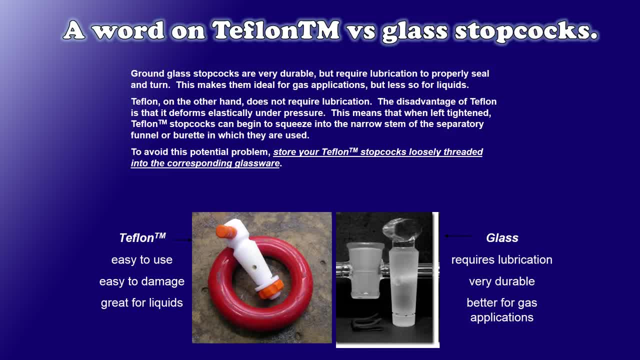 damaged because of how soft they are. So, at the end of the day, be sure that, A- you don't scratch it and, B- that you don't leave your stopcock tightened into your separatory funnel receiver very tightly, because the pressure may actually cause the Teflon to deform. 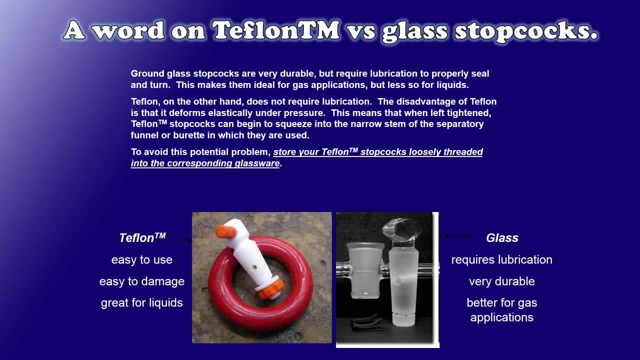 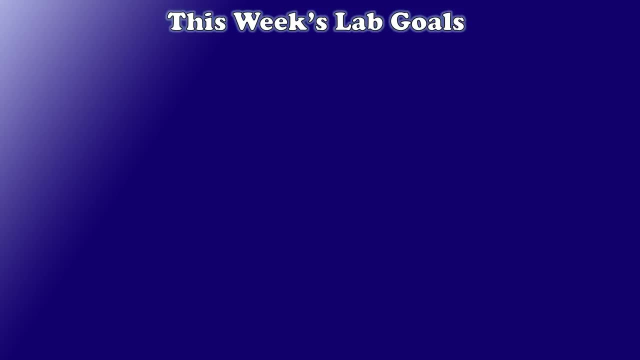 over time. So be sure that you store the stopcocks loosely threaded into the corresponding glassware and not tightly threaded on where they might get deformed. So now that we've covered how and why partitioning of organic compounds happens between two immiscible liquid phases, and the effect that pH can,